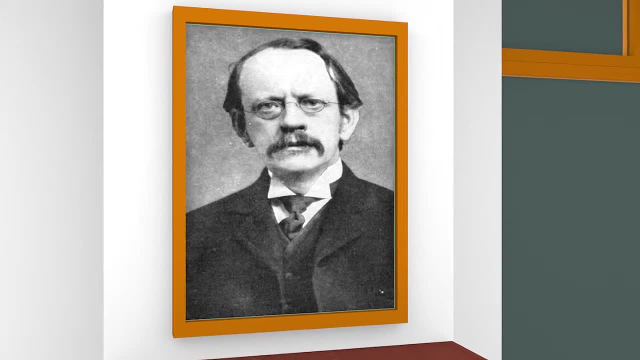 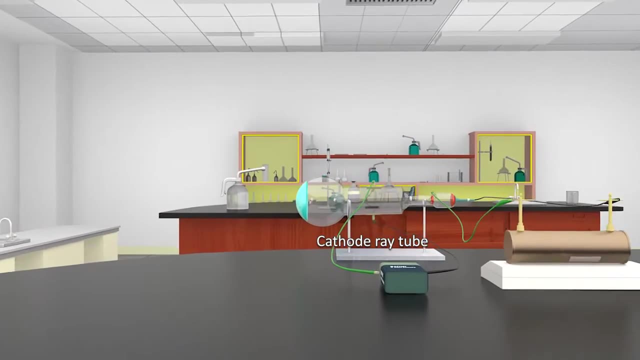 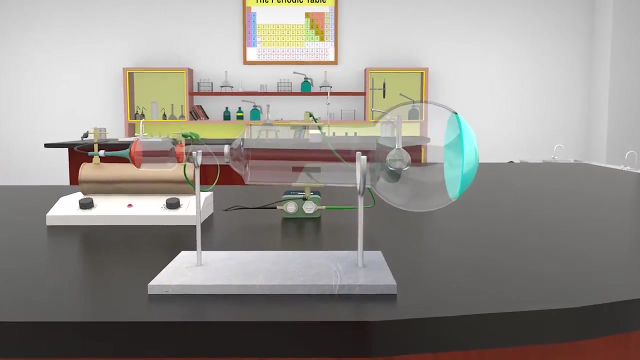 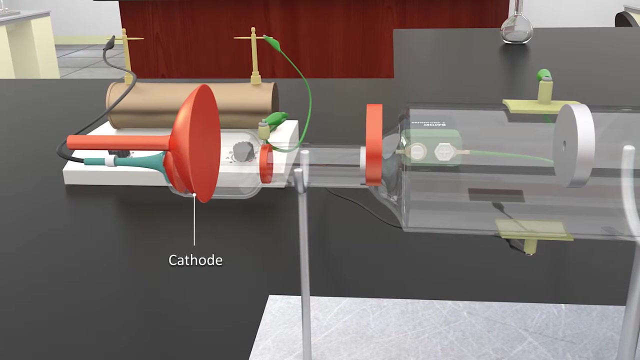 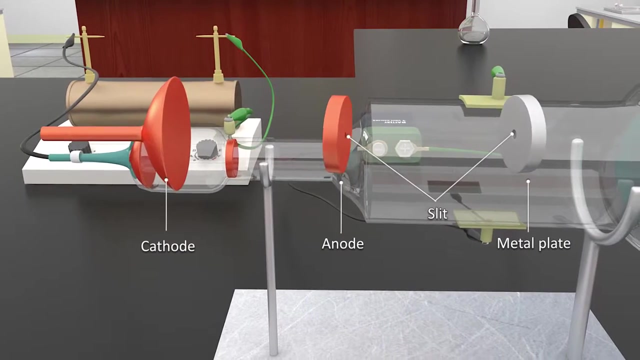 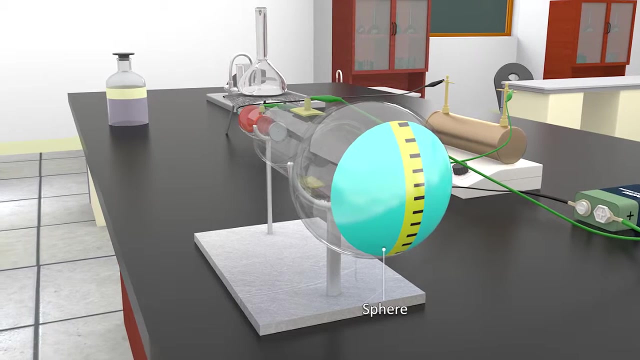 the charge to mass ratio of an electron. The charge to mass ratio of an electron through experiments. The experimental setup included a cathode ray tube With a cathode, an anode and a metal plate. The anode he used the experiment had a slit. At the end of the tube was a large sphere coated with a phosphorescent. 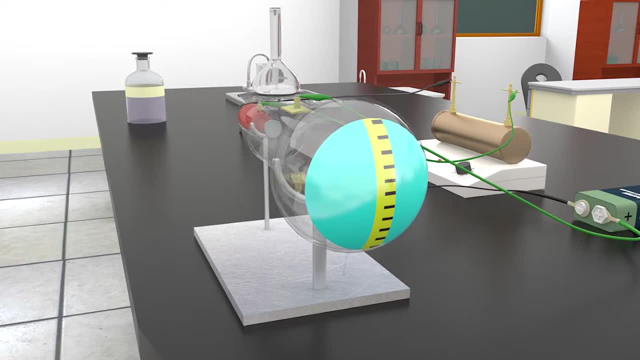 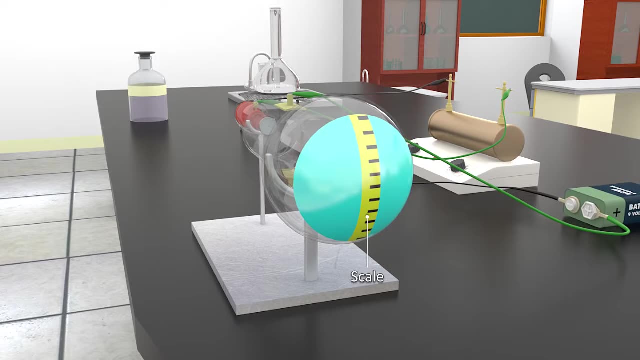 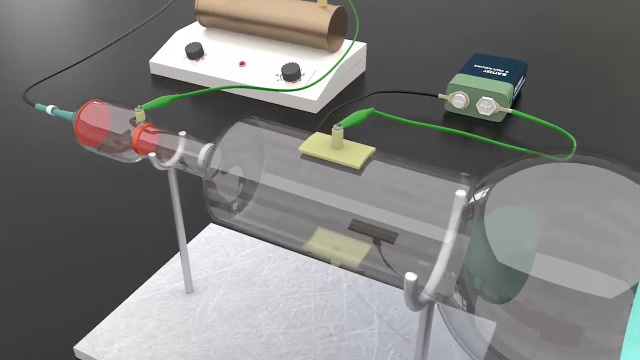 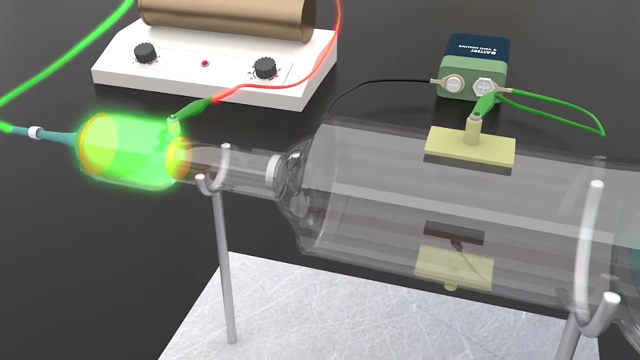 material, so that any beam, after striking it, would leave behind a mark on it. It was also provided with a scale to measure the deflection At high voltage and low pressure. cathode rays were produced in the cathode ray tube In the absence of electric and magnetic fields. the 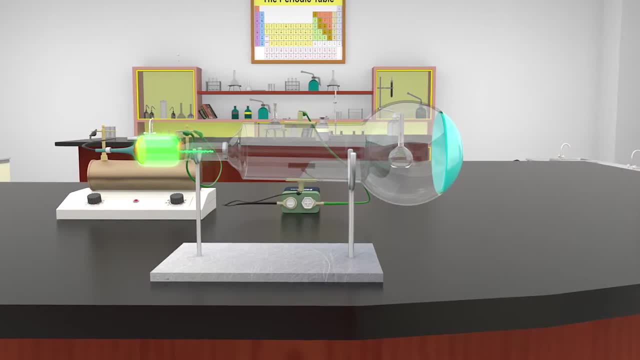 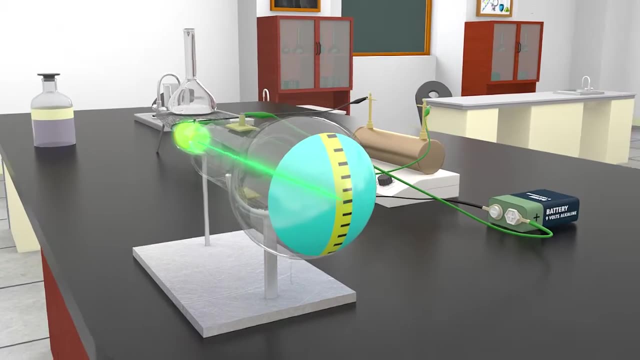 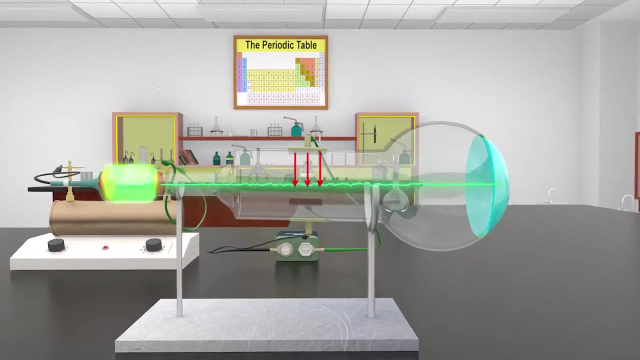 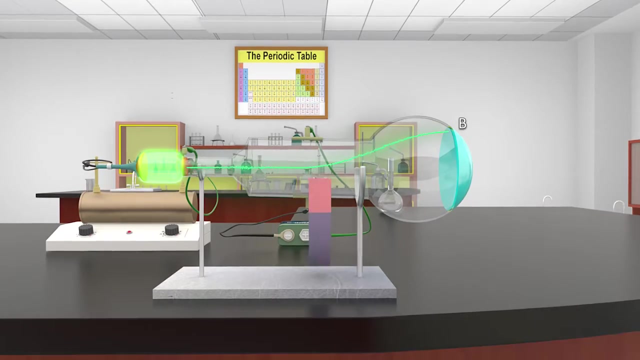 cathode rays produced were found to travel in a straight line without any deflection and struck the tube at point A. When an electric field was applied, the cathode rays were found to deviate from their straight line path and hit the tube at point B. Similarly, when a magnetic field was applied, cathode rays 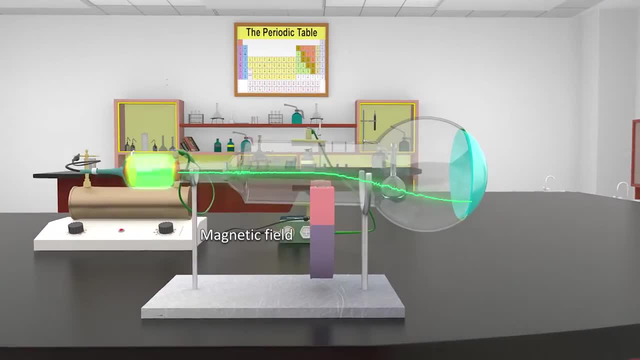 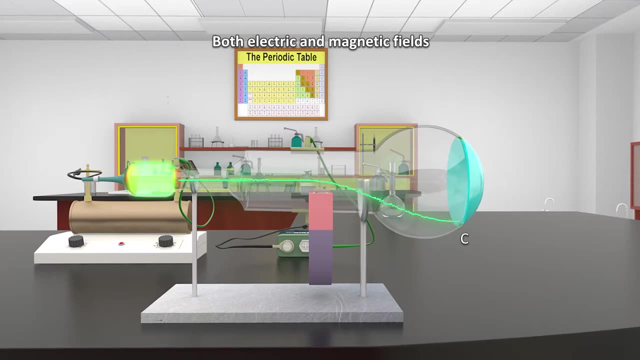 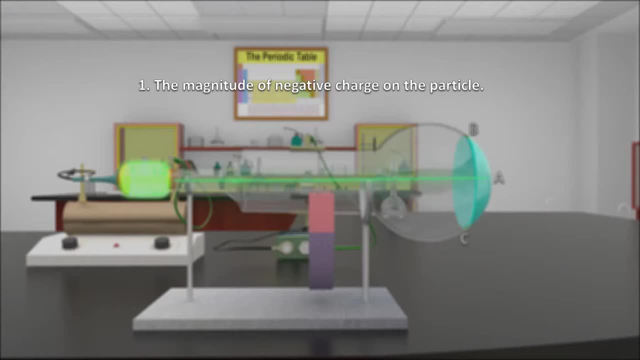 the particle: The greater the negative charge, the greater was the deflection. 2. The mass of the particle: The lighter the particle, the greater was the deflection. 3. The strength of the electrical and magnetic field: The stronger the field. 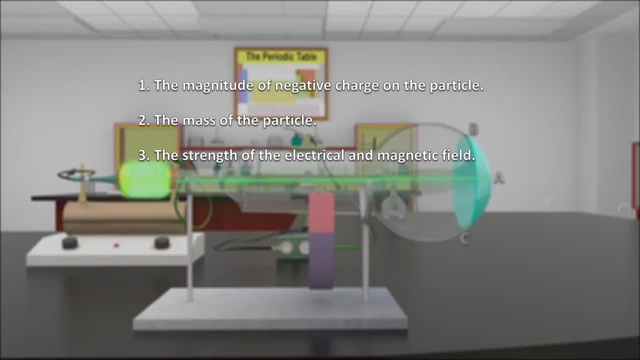 the higher was the deflection. Thompson calculated the charge to mass ratio of an electron by accurately measuring the deflection of electrons when varying strengths of electric and magnetic fields were applied. His efforts culminated in measuring the charge to mass ratio of an electron, which was found to be 1.758820 into 10. the power of 11 coulomb per kg. 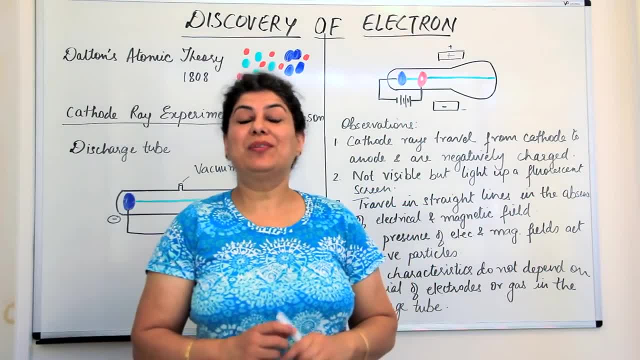 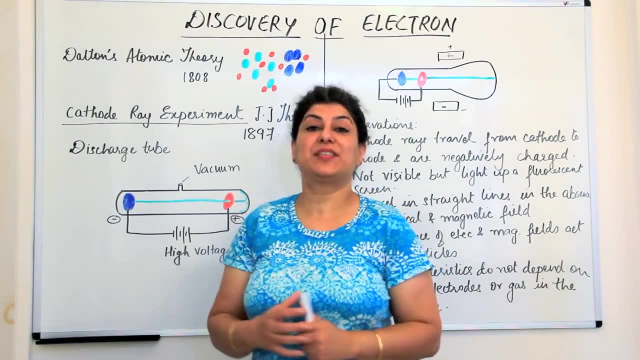 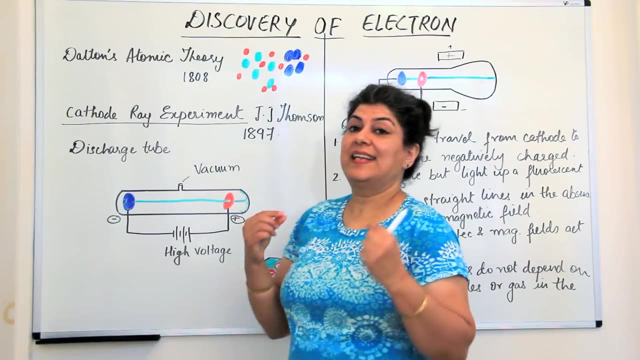 Hello, In this video I'll tell you about the discovery of electrons. In previous videos I talked about the discovery of an atom, how Democritus coined the term atomos and how he said that it was the smallest particle of matter and atomos means it was uncuttable.